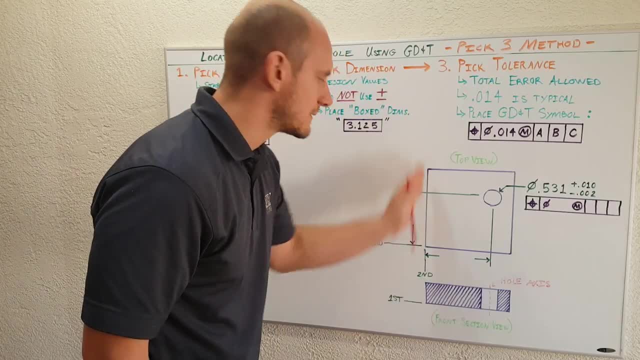 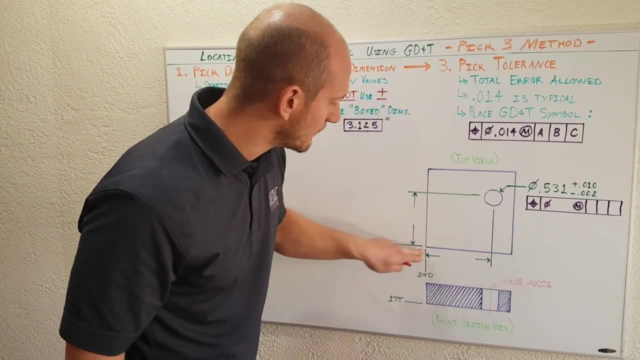 to that surface. Second datum: I'm going to pick this side surface here. It's the surface that I want to locate the hole across from. Third datum: it's this front surface here, or bottom surface, It's the surface that I'm going to locate the hole across from. 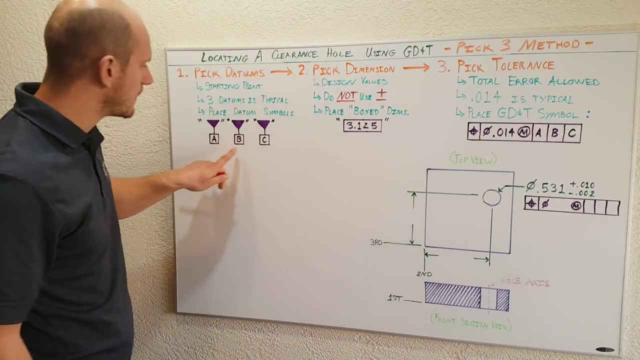 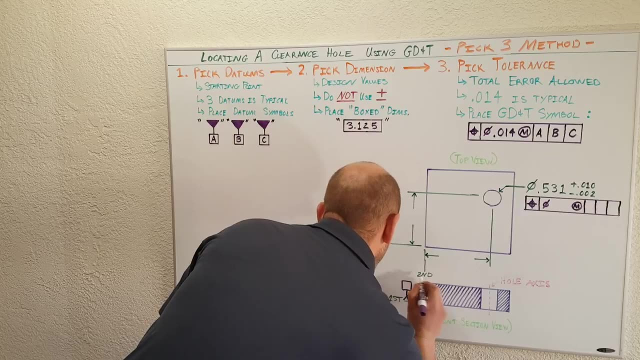 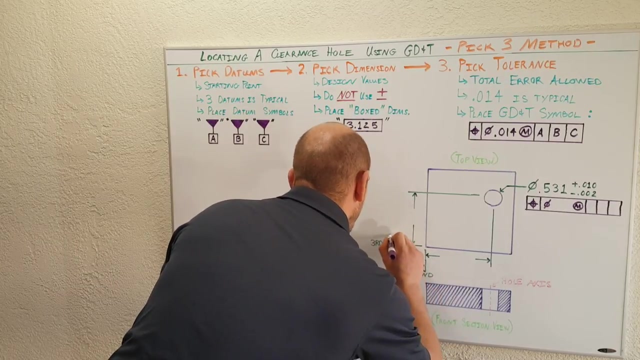 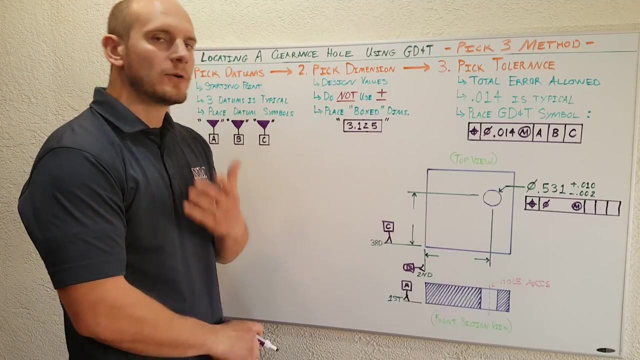 the hole up from. Last thing you want to do: you want to show these datum symbols on your drawing, In that order. Second thing I'm going to do: I'm going to pick your dimensions. They're your design values. You're telling the machinist how far over from your second. 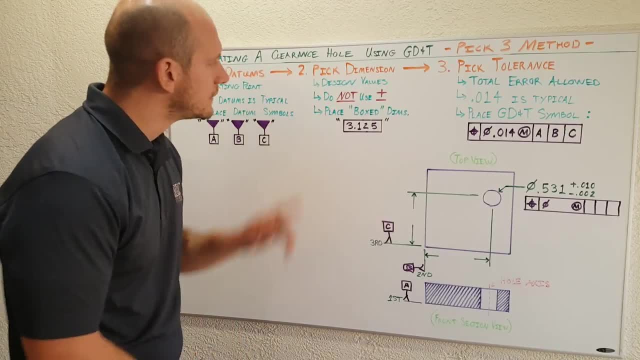 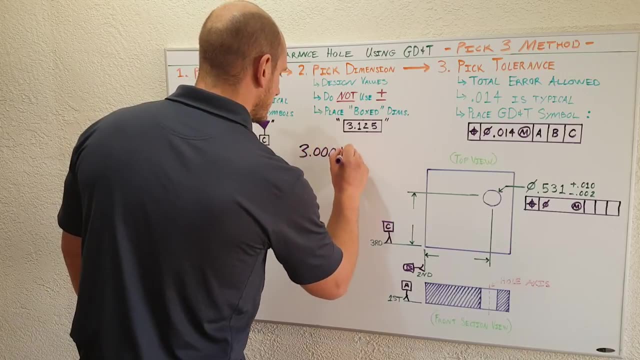 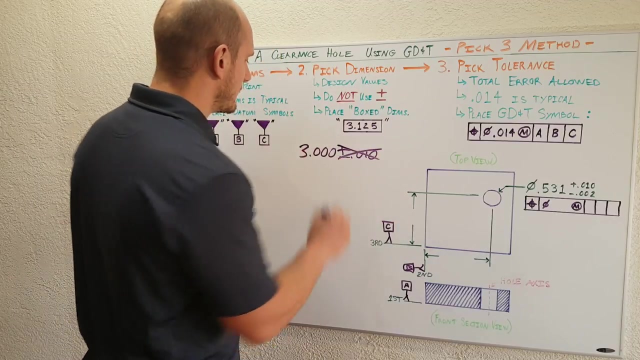 and third datum you want to locate that hole. Do not use plus or minus dimension that you typically see on drawings. So what you usually see is something similar to this: Do not do this. Drop the plus and minus off that Then box your dimension. 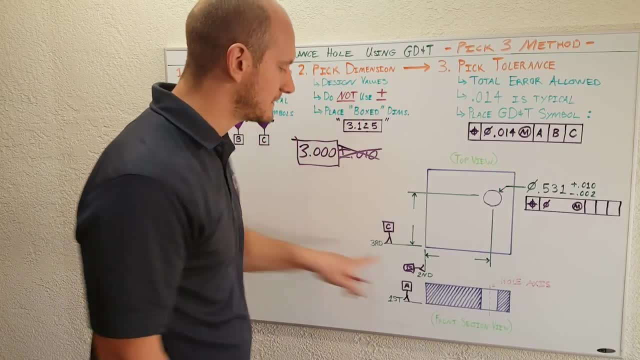 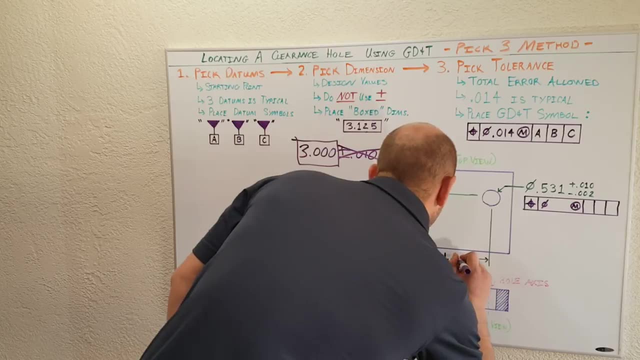 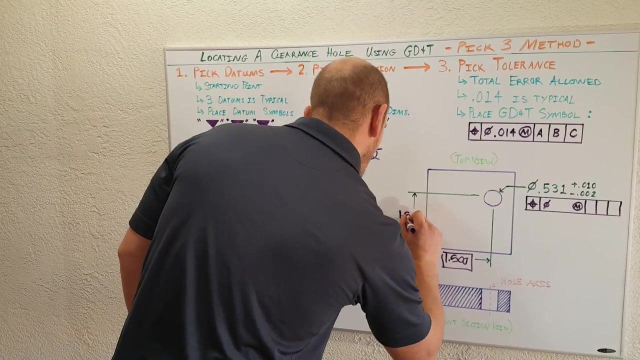 Now take your dimensions, your design values and place them here in this location, in this location. so the machinist knows how far to locate that hole from your datum: One and a half inches boxed, One and a half inches boxed, And now he knows one and a half. 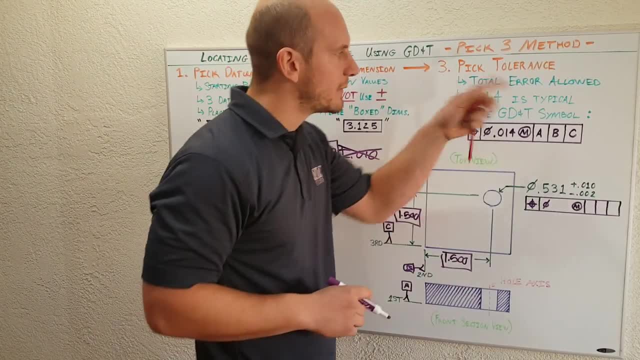 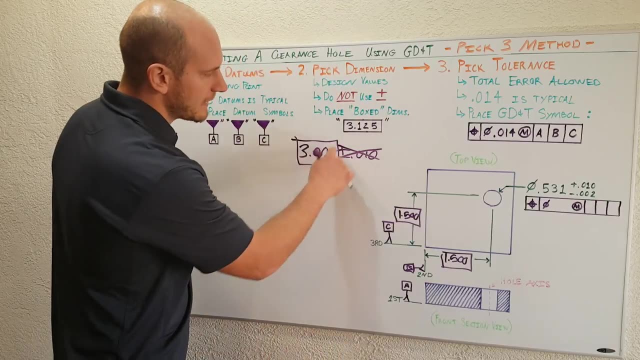 inches over one and a half inches up. Third thing you're going to do: you're going to pick your tolerance. Your tolerance is how much you're allowing the machinist to be off when he or she drills this hole. Notice, we eliminated your tolerance here, so we have. 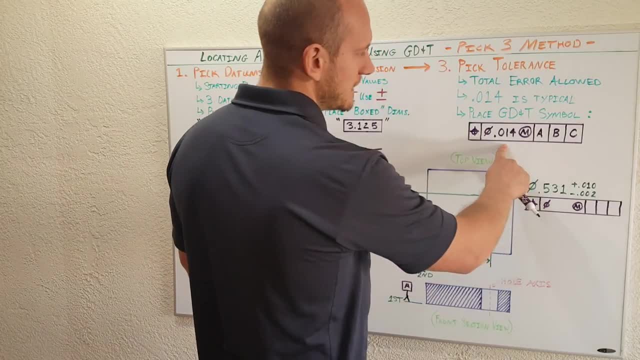 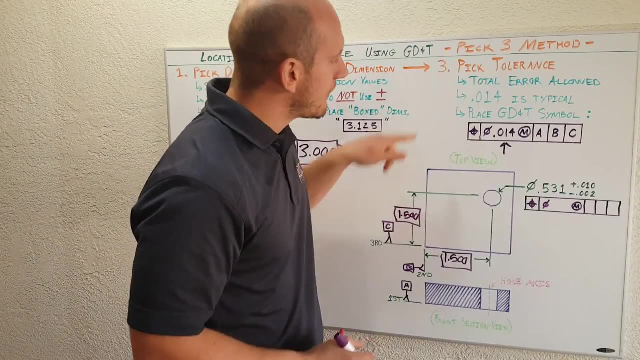 to place it somewhere, And where we place that is inside the GDMT symbol right here. Typically in industry, you'll see 14 thousandths. What you now want to do is you want to take this GDMT symbol that I've generated for you here and just simply place that underneath. 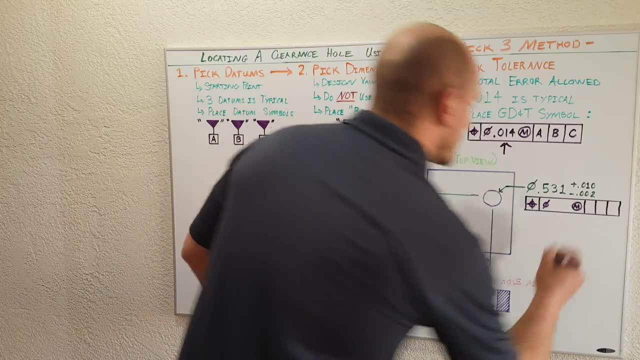 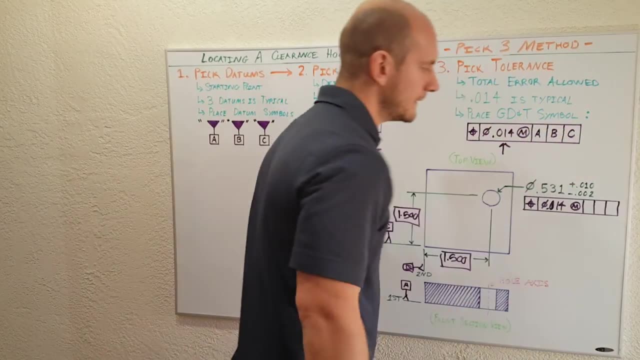 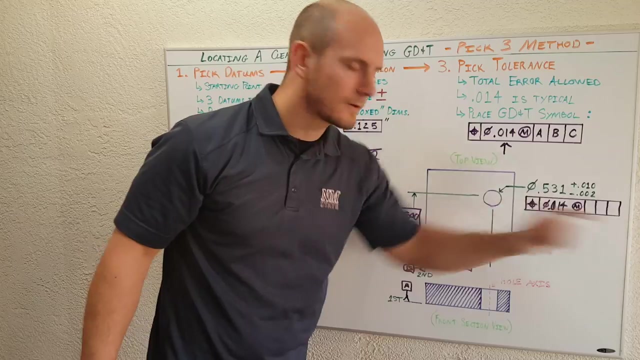 your size and your size tolerance for that hole. So I'm going to take that write in my 14 thousandths. Then you're going to take your datums in order: A, B and C- first, second, third- and you're going to place them in order inside your GDMT symbol. So you're